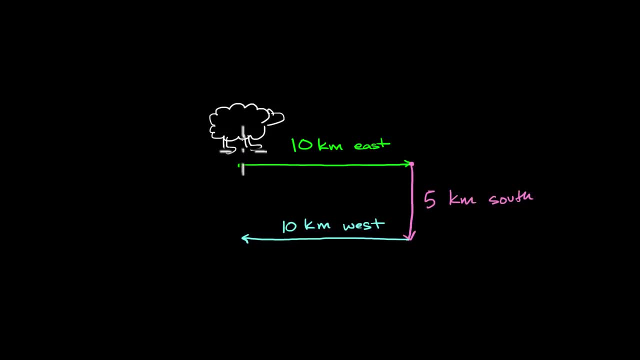 And pause the video and think: pause the video and see if you can figure that out. How far has that sheep traveled? All right, now let's try to answer this together. And it's a little bit of a trick question because, depending how you interpret the idea, 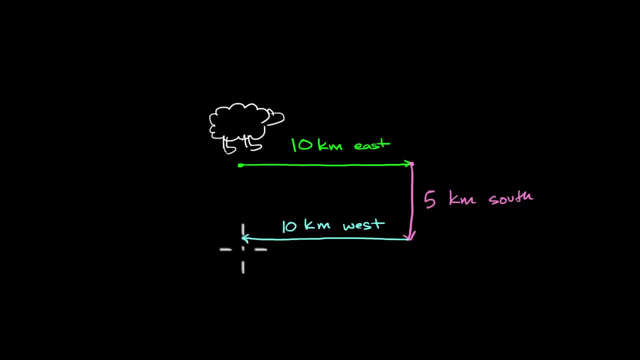 how far something has traveled. there could actually be two valid answers here. One answer is: you could say what is the total distance traveled. So let me write this one down. This is an important concept: Distance Traveled, Traveled. 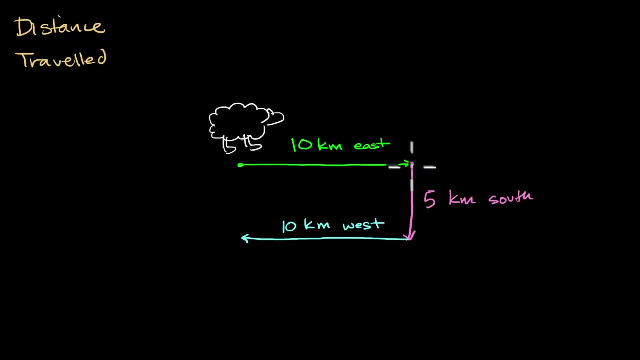 And this would be the total length of its journey, or the total length of its path. So the distance traveled in this situation would be 10 kilometers plus five kilometers, Plus five kilometers, Plus 10 kilometers, Plus 10 kilometers, Which would give us 25 kilometers. 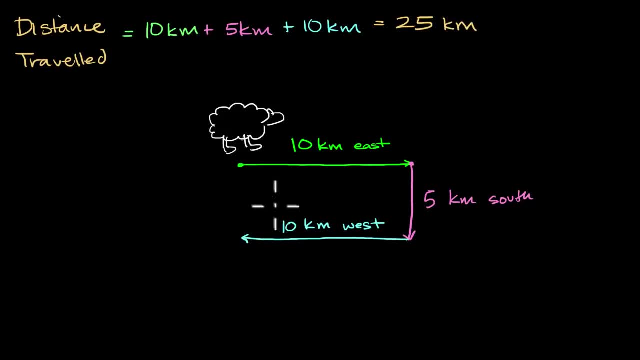 That would be 25 kilometers. So some of y'all might have said that the sheep traveled 25 kilometers. If that's what you came up with, what you calculated is the total distance traveled. Now some of you might have said: wait, hold on a second. 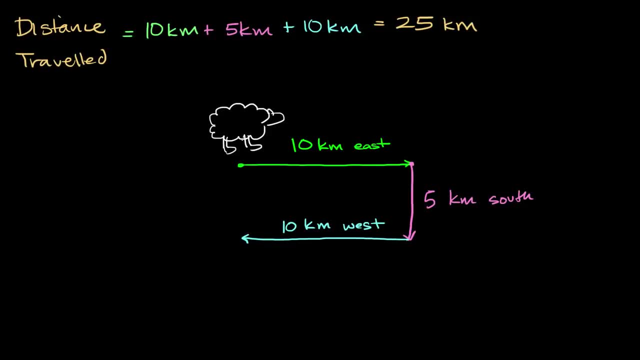 The sheep was here before, and then it ends up right over here at the end of its journey, And so its change in position is it would have moved a net five kilometers south from this point to this point, which would have been five kilometers south. 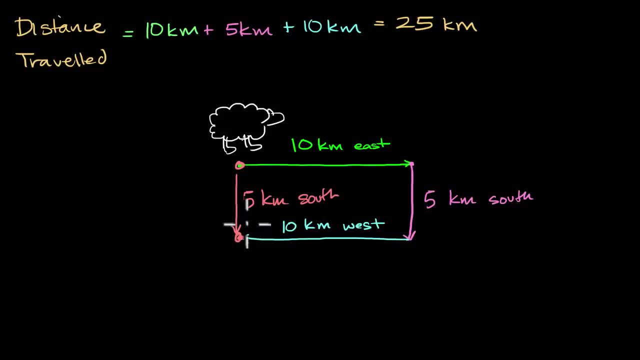 It doesn't matter what it did along the way, what its path was. At the end of the day, it ended up five kilometers south of where it started out- And this would also be a valid way of saying how far it traveled- And this notion is known as displacement. 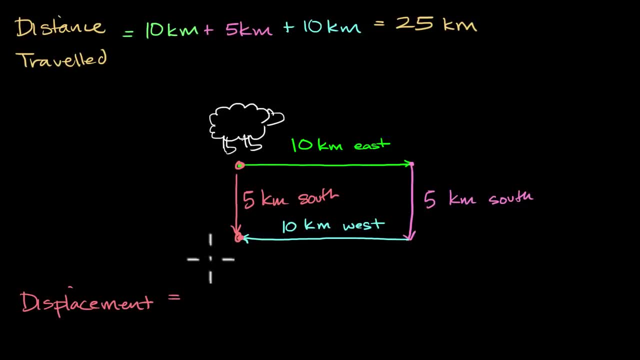 So the displacement would be, in this situation, five kilometers south. So pause this video. What do you think is the definition or the difference between saying the distance something traveled versus its displacement? Well, as we mentioned, the distance something travels is the entire length of its journey. 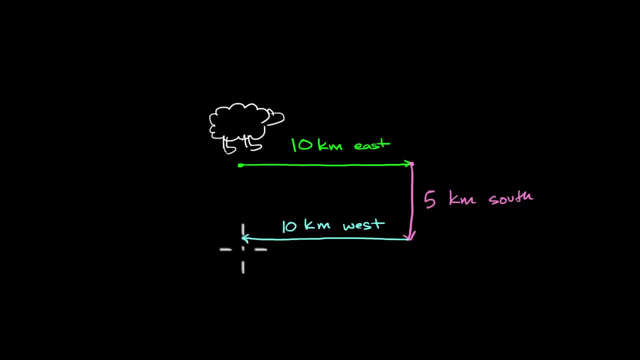 how far something has traveled. there could actually be two valid answers here. One answer is: you could say what is the total distance traveled. So let me write this one down. This is an important concept: Distance Traveled, Traveled. 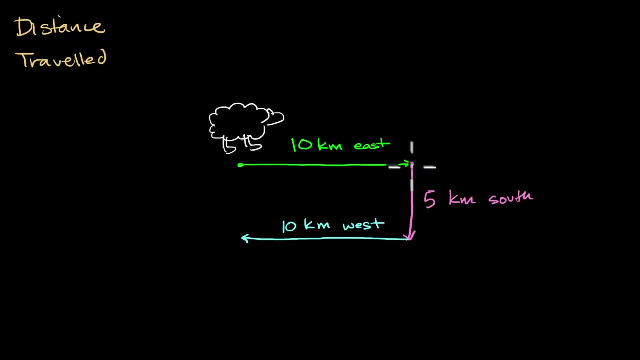 And this would be the total length of its journey, or the total length of its path. So the distance traveled in this situation would be 10 kilometers plus five kilometers, Plus five kilometers, Plus 10 kilometers, Plus 10 kilometers, Which would give us 25 kilometers. 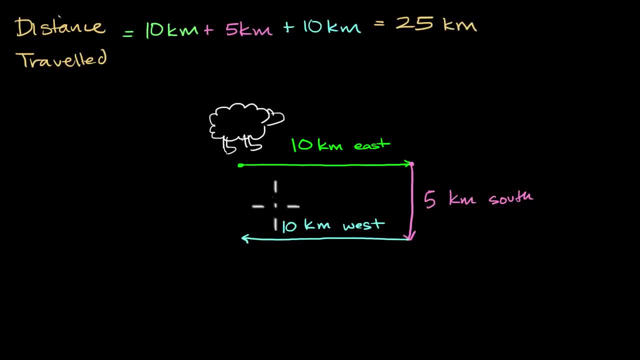 That would be 25 kilometers. So some of y'all might have said that the sheep traveled 25 kilometers. If that's what you came up with, what you calculated is the total distance traveled. Now some of you might have said: wait, hold on a second. 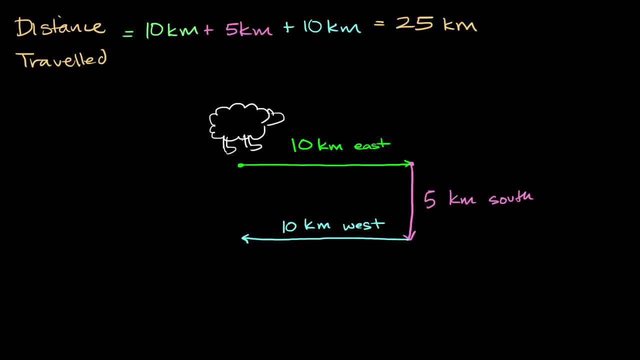 The sheep was here before, and then it ends up right over here at the end of its journey, And so its change in position is it would have moved a net five kilometer south from this point to this point, which would have been five kilometers south. 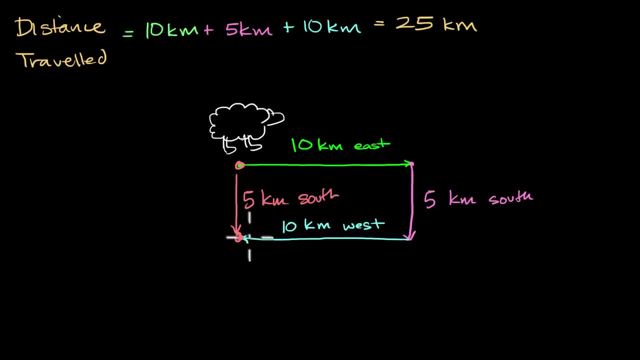 It doesn't matter what it did along the way, what its path was. At the end of the day, it ended up five kilometers south of where it started out- And this would also be a valid way of saying how far it traveled- And this notion is known as displacement. 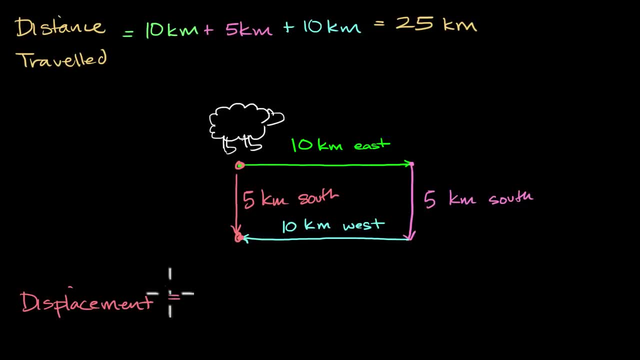 So the displacement would be, in this situation, five kilometers south. So pause this video. What do you think is the definition or the difference between saying the distance something traveled versus its displacement? Well, as we mentioned, the distance something travels is the entire length of its journey. 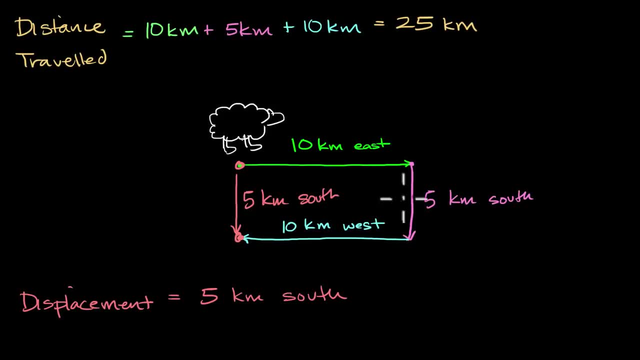 It's the entire path And this thing will never be negative. You could travel zero kilometers, but as long as you are, you're not going to be traveling. As long as your position keeps changing, this thing will only increase, because it's the total length of your path. 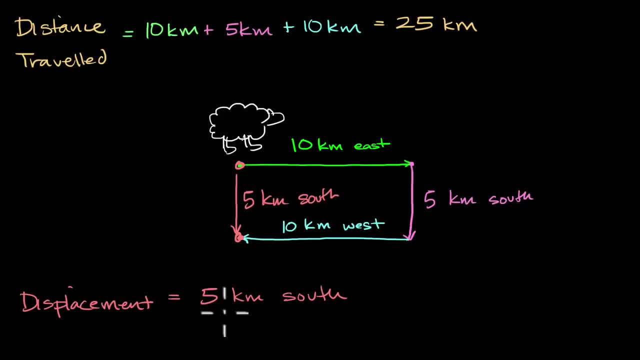 Your displacement is your change in position. And since it's a change in position, not only will we mention the five kilometers, we'll say in what direction. The position of the sheep has changed: five kilometers to the south. So let me write this down. 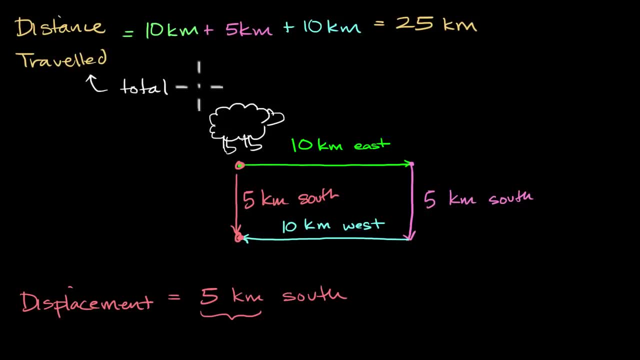 This is total length of path. total length of path. The total length of path is the distance traveled, while the displacement is the change in position. Change in position. 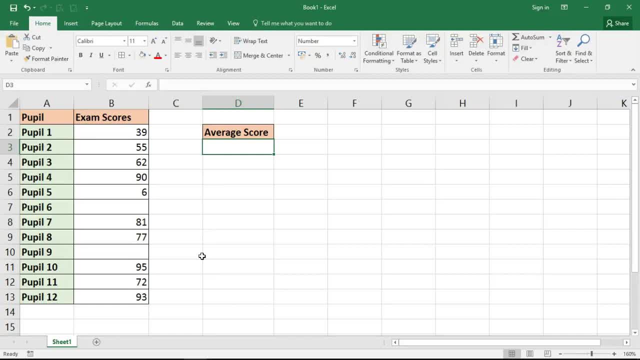 Hello and welcome to this video tutorial from ComputerGarGarcom. In this video we are going to look at how to calculate the average by excluding outliers in the range. So I have these exam scores on this spreadsheet and I want to know where the average score is. 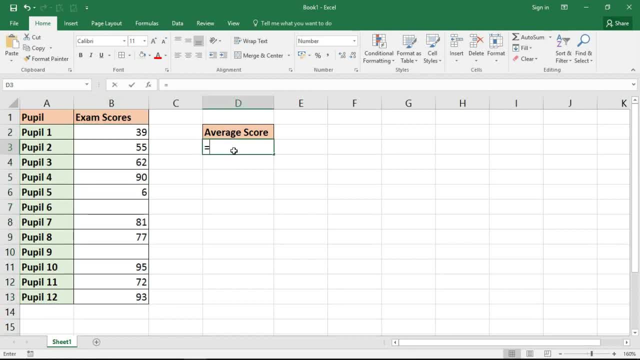 Now I could proceed and use the typical average function and if I do that right now, on these exam scores I receive the result of 67. But that result is being distorted somewhat by pupil 5's exam score. The fact that that pupil only got a 6 is very much outside the. 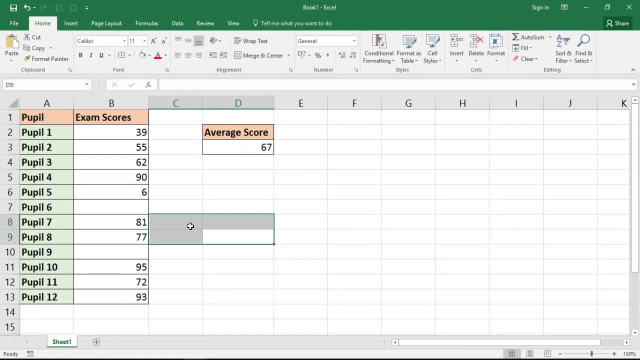 normal exam score range and that is affecting the average. So an alternative is that I could use a function called trim, Trim, mean, and this will also provide me with the mean average, just like the normal average function, but will give me the opportunity to exclude outliers in that range. So values. 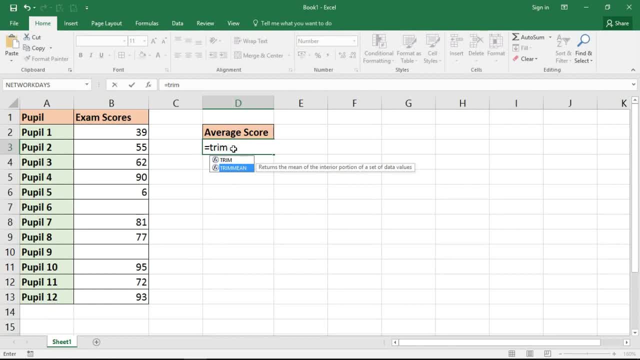 that are either excessively low or excessively high, And I get to choose. when I use the word excessive, I get to choose how much of those outliers to exclude. And here we go. if I proceed with the trim mean function, I'm prompted first of all for the array, and that is the range of cells we're testing.